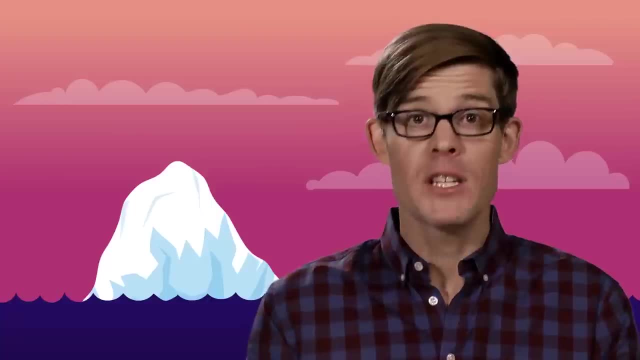 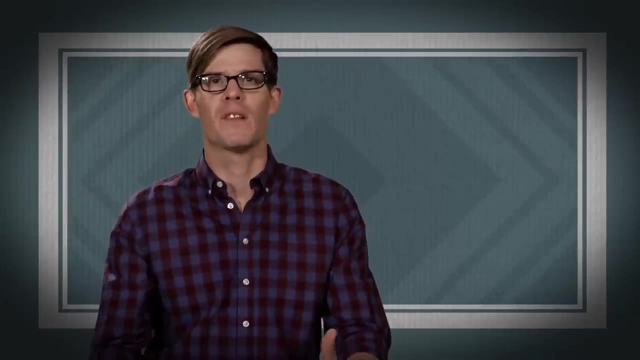 Let's not beat around the rapidly melting iceberg here. Climate change is happening and we are causing it. The evidence is overwhelming. Scientists usually reserve this level of agreement for claims like Earth is a planet or air is real. Yet here we are: The climate change. 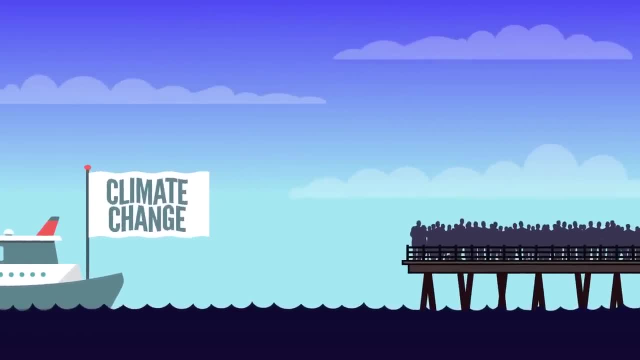 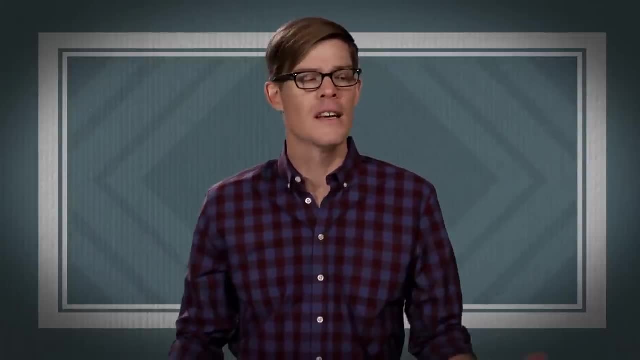 ship has now left the dock, yet lots of people on shore are still debating whether boats can actually float. But maybe you're a person who trusts and accepts what climate scientists are telling us. It's just sometimes it's hard to explain why. I mean, we've all 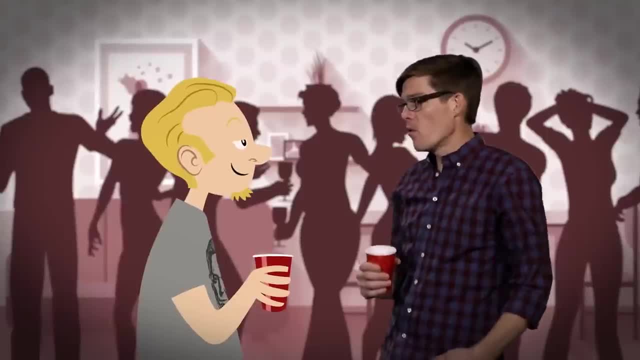 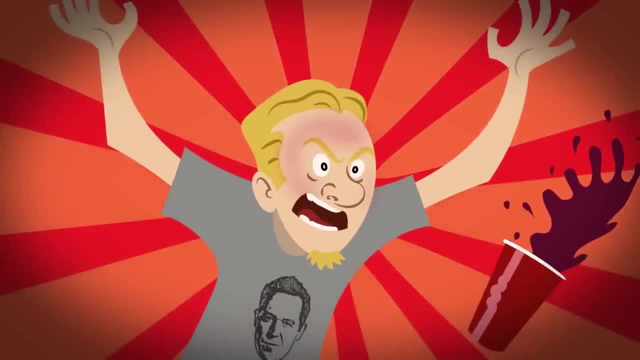 been there. I mean, I care about the environment. I figure, with the polar bears and everything, we might as well try electric cars. What do we have to lose? And then they go- caps lock, serious, saying they have proof that climate change is a hoax perpetuated by scientists. 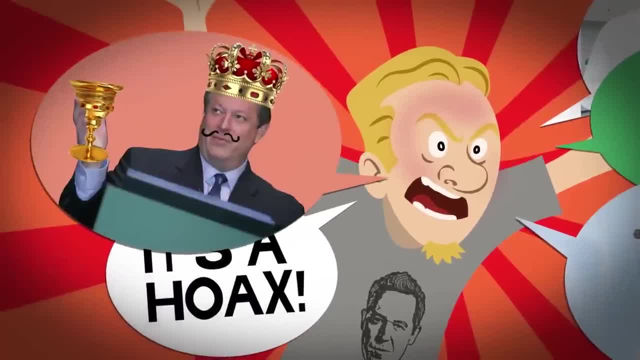 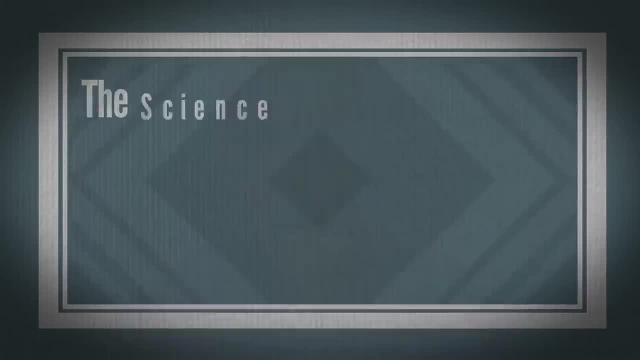 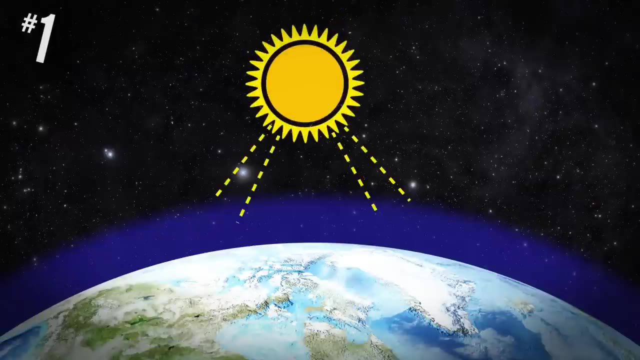 paid off by the polar bear lobby as part of a plan to install Al Gore as supreme world polar bear emperor. Wake up sheeple. To keep that from happening, we put together this handy reference: The sun is the source of warmth on Earth, so thanks for that sun. Ice and clouds reflect. 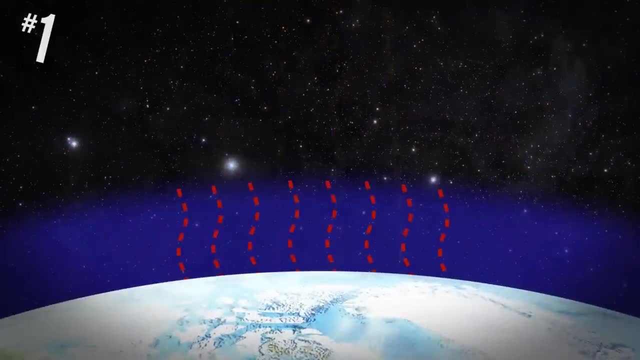 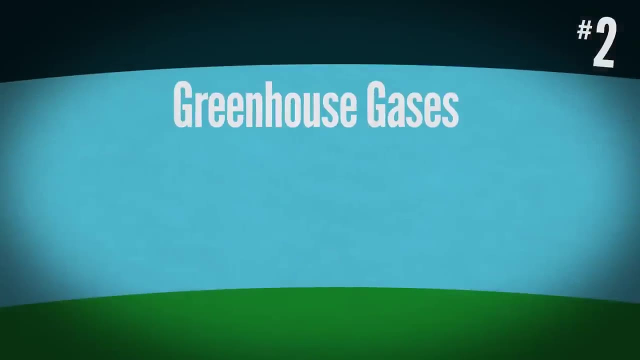 some of its light away, but the rest is absorbed by land and water and re-emitted as heat. Some of that heat escapes to space and some is held in by the atmospheric greenhouse effect. The insulating effect of Earth's greenhouse gases are the reason that life exists as we. 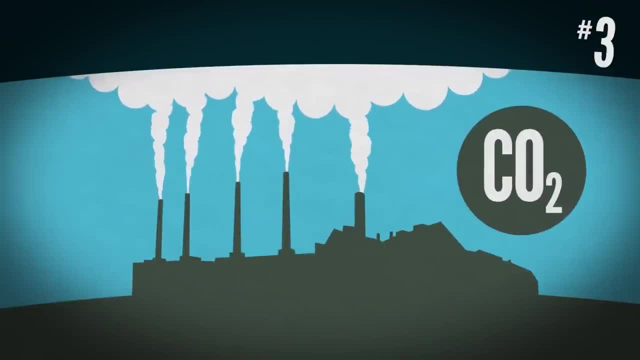 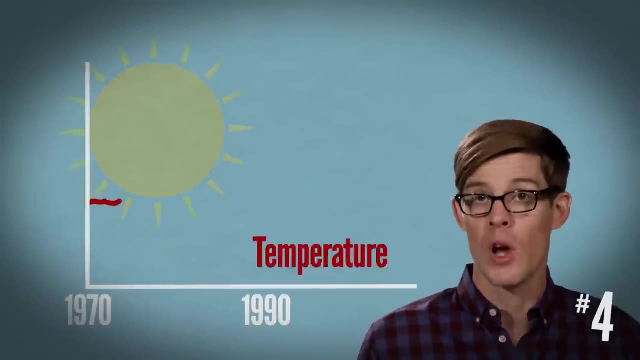 know it, but human activities have increased the concentration of one of them, carbon dioxide, 40% since the industrial revolution. We know the sun's output has varied during history, but since the 1970s, the period when global temperatures increased the fastest temperature. 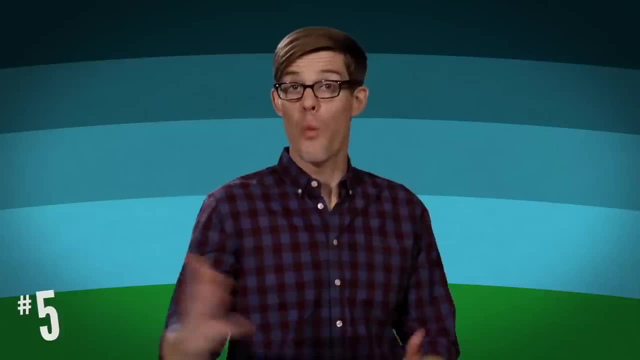 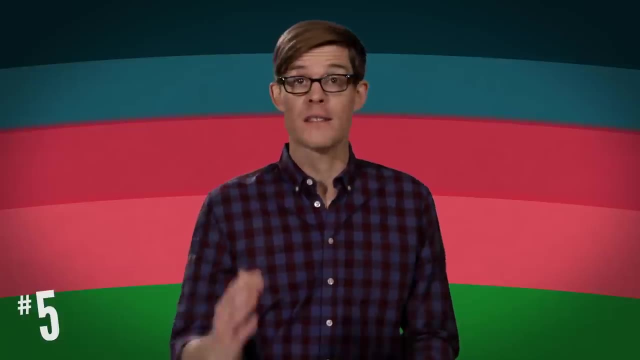 and solar activity have moved in opposite directions. If the sun was to blame, it would cook the upper and lower layers of the atmosphere together. Instead, we only see warming in the lower layers, the same place that human greenhouse gases like carbon dioxide are piling. 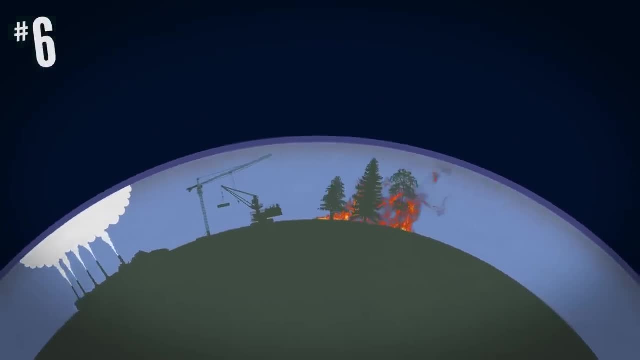 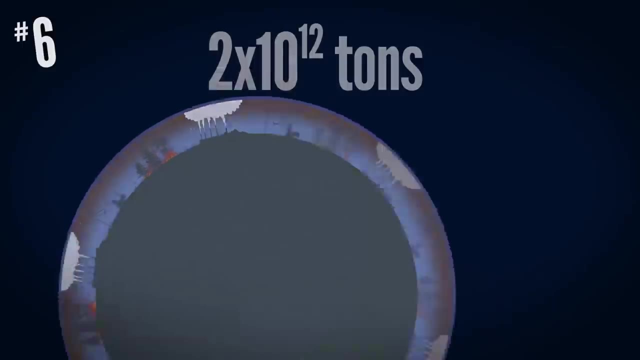 up Since 1870,. with fossil fuels, cement production and land use combined, humans have put about 2,000 gigatons of CO2 into the atmosphere. That's two million million tons, and about 40% has stayed there. 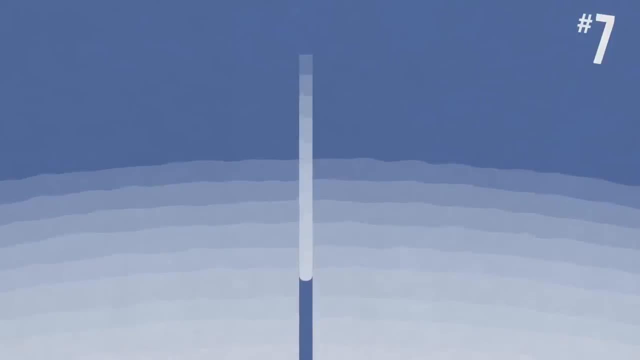 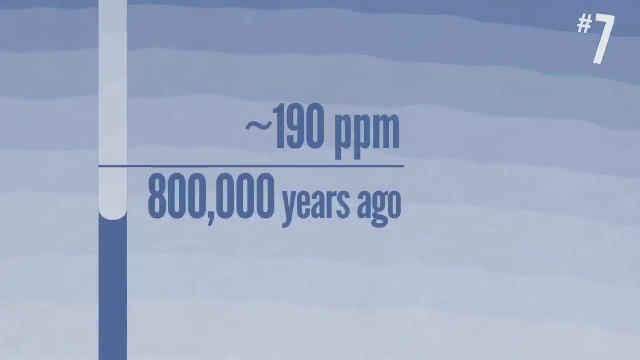 Studying gases trapped in ice cores has let us see what Earth's atmosphere was like in the past. At more than 400 parts per million, today's carbon dioxide levels are the highest they've been for almost a million years, That's before humans even existed. 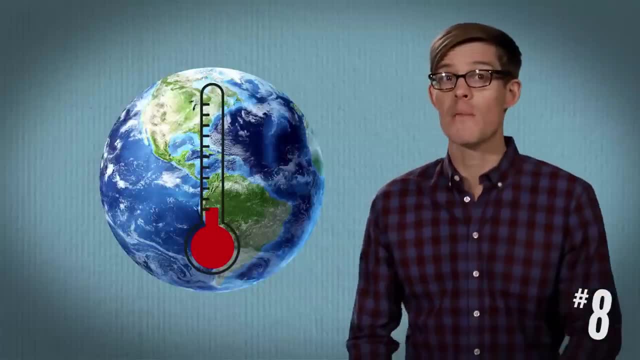 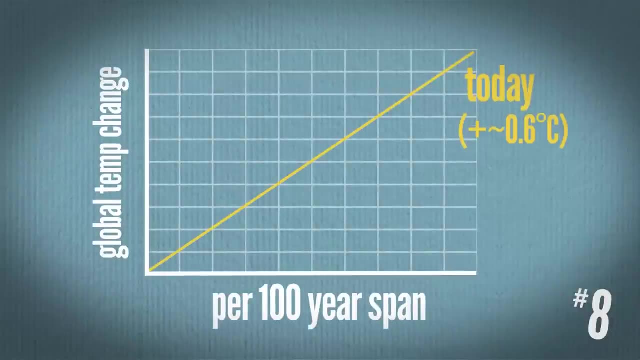 Totally uncharted territory for us. More carbon dioxide in the atmosphere means average temperatures across the globe are increasing, And fast. Right now, Earth is warming about 10 times faster than at the end of an ice age. Okay, so CO2's increasing. How do we know it's our fault. 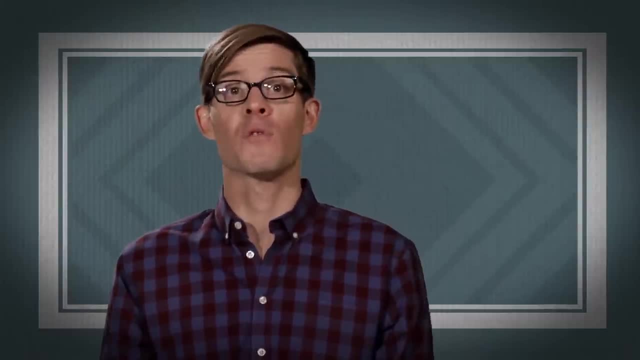 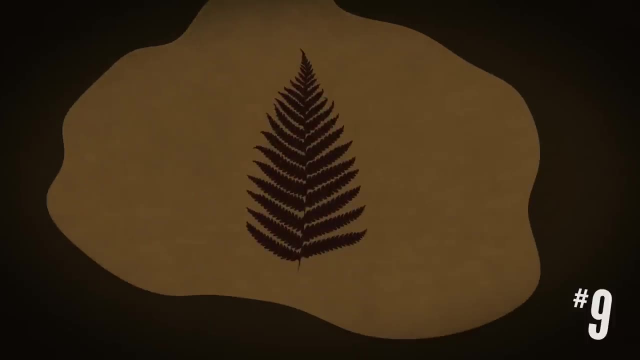 Well, we know that the temperature of the atmosphere is increasing and that's because we know it's our fault. The best evidence comes from looking at what isotopes, or different kinds of carbon, are in the atmosphere. Fossil fuels come mainly from old plants. Plants prefer to use the lighter isotope. 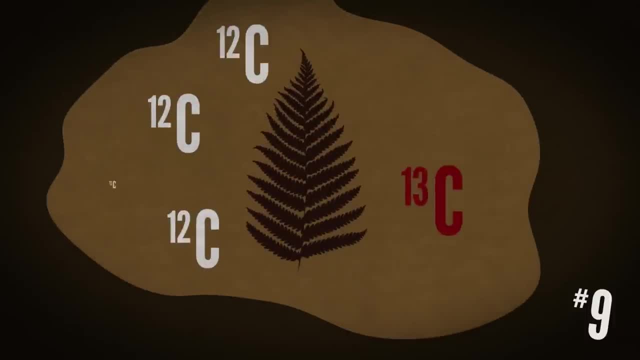 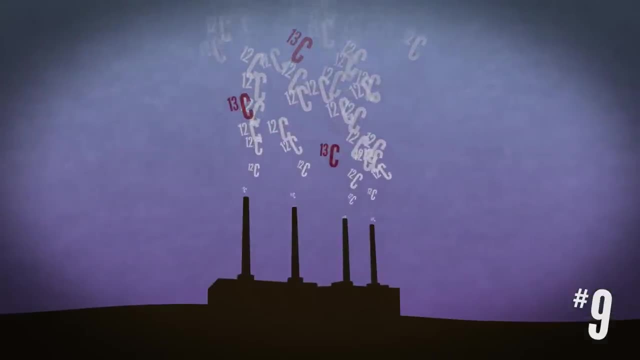 carbon-12, over the heavier carbon-13,, so they contain a higher ratio of 12 to 13 than the atmosphere does. When more fossil fuels get burned, the percentage of carbon-12 in the atmosphere should go up, and that's exactly what we see. 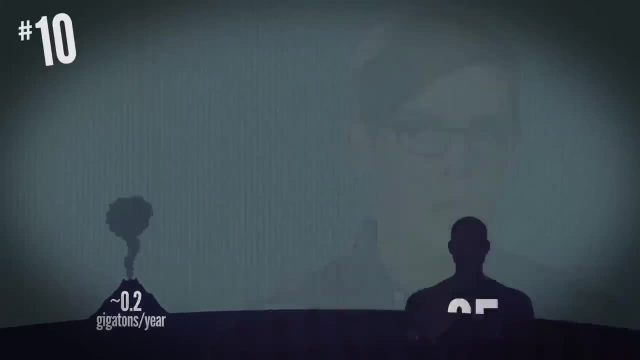 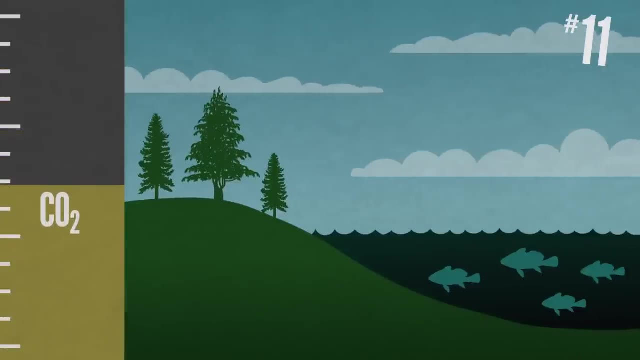 And it's not because of volcanic activity. Volcanoes only emit about 1% as much CO2 as we do. We know that CO2 is balanced in exchange between the atmosphere, plants and animals, but eliminating carbon sinks has released centuries worth in just a few years. 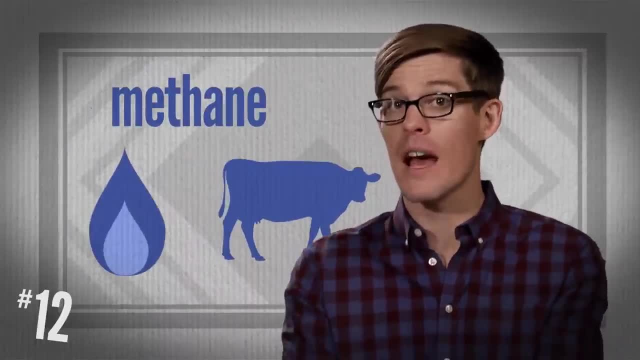 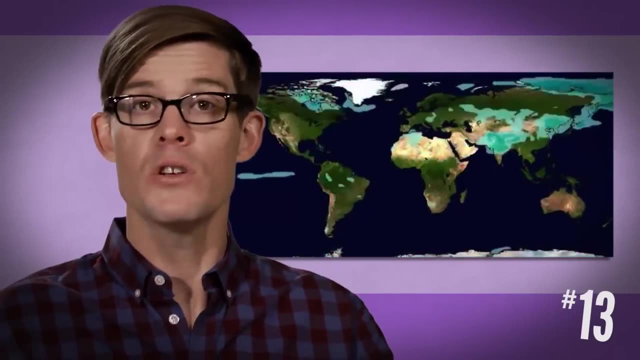 Other greenhouse gases are also increasing, like methane from farm animals and natural gas processing or nitrous oxide from fertilizers. If we run simulations just using natural causes of climate change, they predict no change or even cooling in the 20th century, And that. 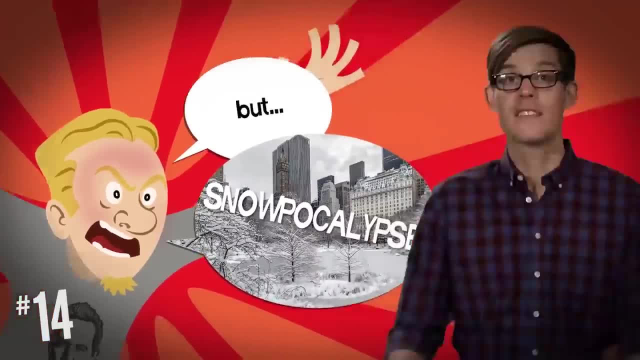 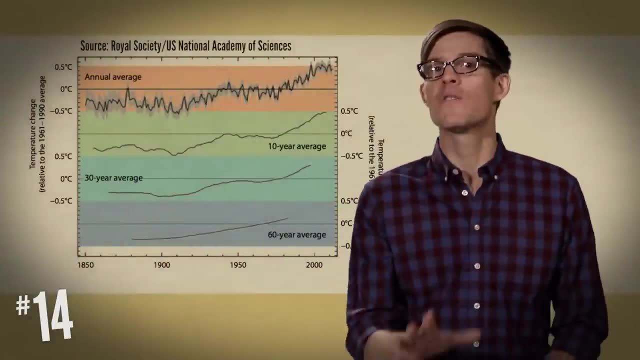 is not what's happening. It's still going to get cold in some places, but in the 2000s there were twice as many record highs as record lows, And each of the past three decades has been warmer than any other decade since we started measuring in 1850.. 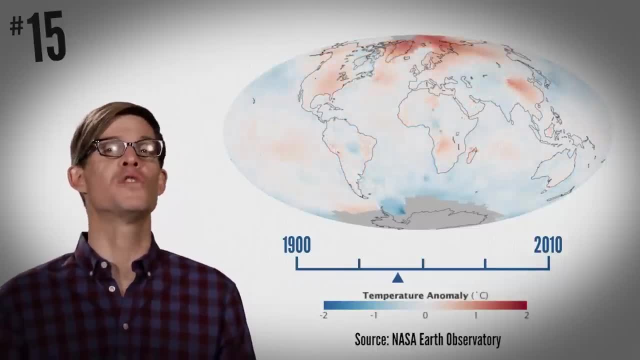 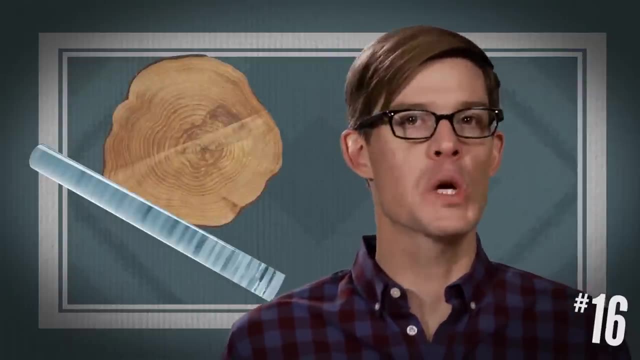 Since 1900,, actual temperatures around the world have increased almost a full degree, and most of that has happened since the 1970s. Looking at data from tree rings and ice cores, the past 30 years is probably the warmest in eight centuries. Of course, not every place. on Earth warms equally. Oceans cover more than 70 percent of Earth and they absorb more than 90 percent of the Earth's temperature, And that's because of the fact that the temperature in the oceans is higher than 90 percent of the heat added to the planet Naturally. 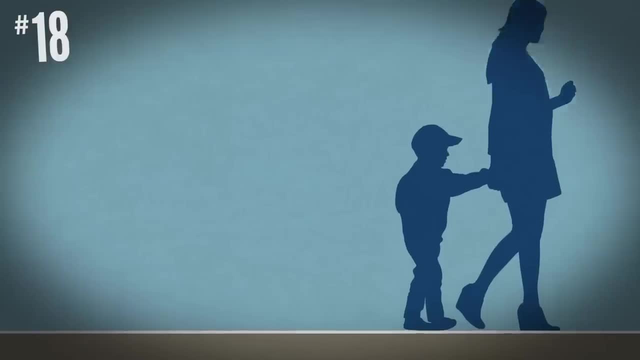 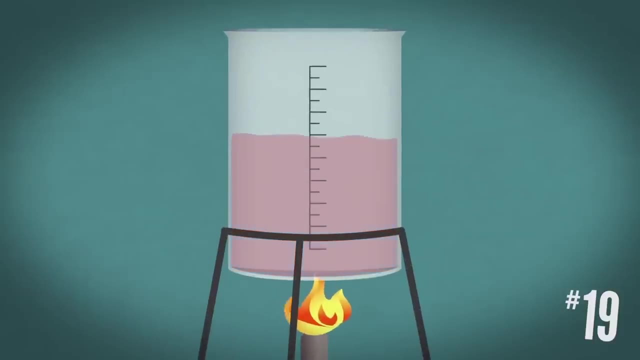 that's where we see the most extreme changes Around the world. oceans are rising a tenth of an inch per year and they're up 8 inches since 1901. This is because water expands as it warms And when ice sheets in glaciers. 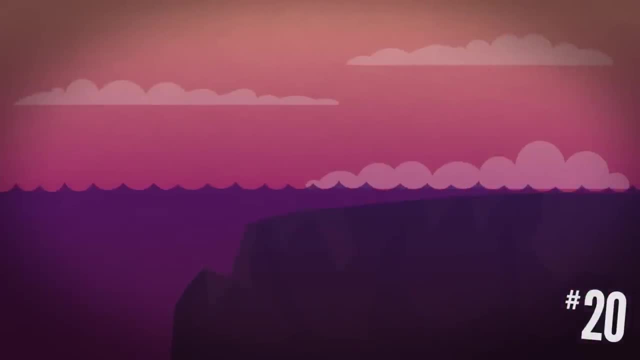 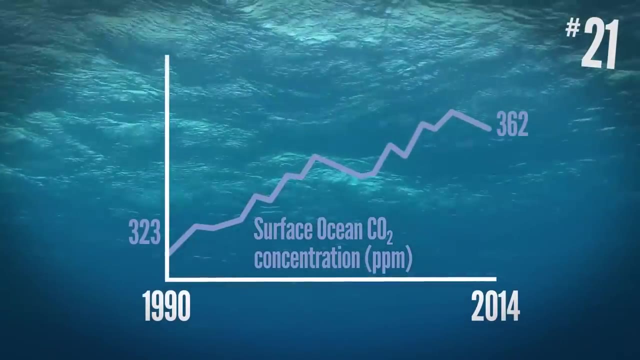 melt in Greenland and Antarctica, water that's normally on frozen land gets put in the ocean. The oceans are Earth's largest carbon sink. As more CO2 enters the atmosphere, more of it dissolves in the ocean, which makes the water more acidic. This doesn't mean the